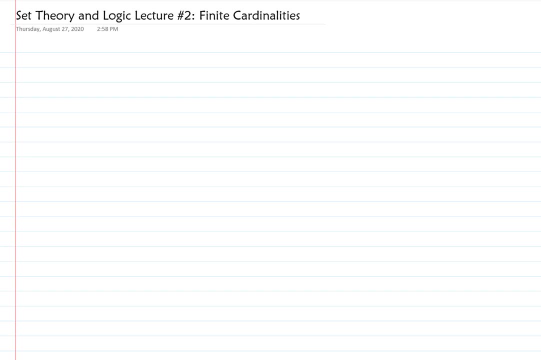 Unless there's infinitely many things in the set. then it gets a little bit more complicated And we're going to ignore that complication today. We're only doing finite cardinalities, Okay, so that means you can look at the set and simply count how many things are there, and that would be the cardinality of the set. Okay, so let me do this. We'll just start off really simple. 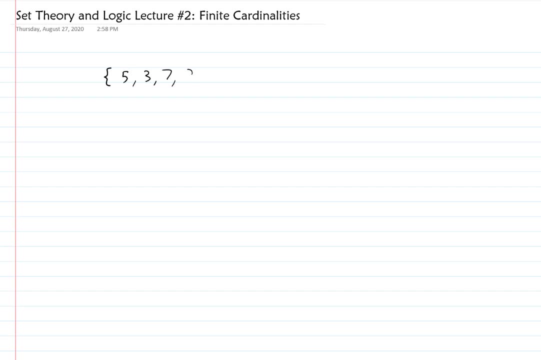 Let's look at that set, Okay, and I want to know the cardinality of that. Remember, the symbol we're going to use, for cardinality is identical to the absolute value symbols. So I could do that And what would be the answer? How many things are in that set? I see five, So that's the answer. 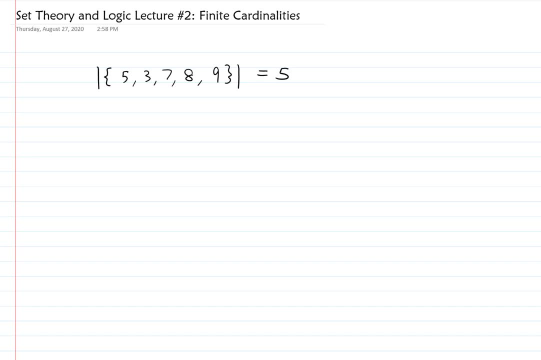 Okay, another way to do it, just so that you know, is I could have given that set a name and said a equals that, And then I could have written the cardinality of a equals five. Okay, All right, let's go back to the way it was. 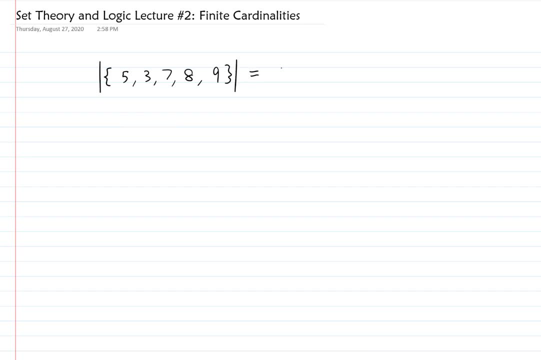 Okay, Now it's a pretty simple concept, I think, right, Do you agree? But there are some small technicalities that are very, very common for confusing people. at first It's very easy to get past this confusion and then it will probably never confuse you again. Okay, but probably the first time it will. 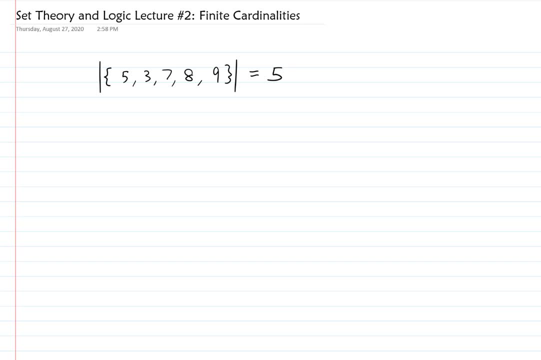 And all we need to do is just point out the possible confusion and get you past it once, and then it'll be fine. Okay, Look at this. I'm going to take a set, Okay, And inside of that set I'm going to put a set that has, let's say, the numbers one half. 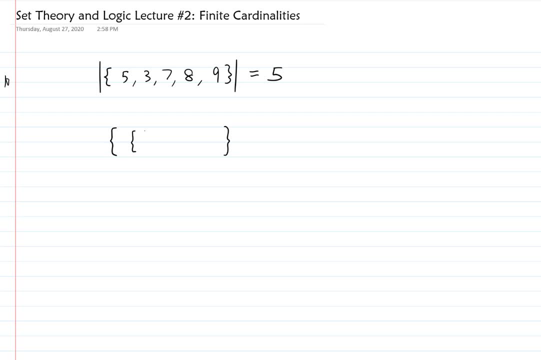 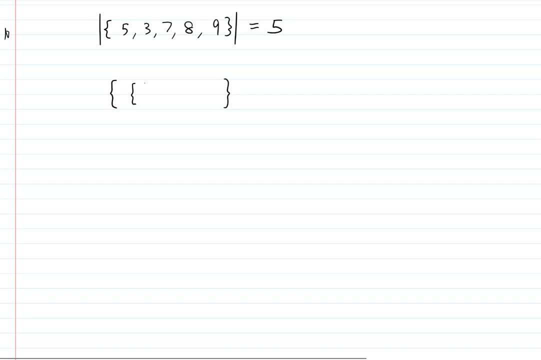 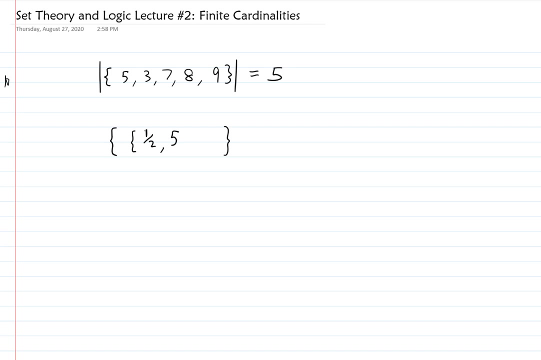 My pen's not working. What's going on here? Give me one second There. that fixed it. Okay, let's say one half and five And pi? How about that? So I have a set, and inside that set is another set that has three elements. 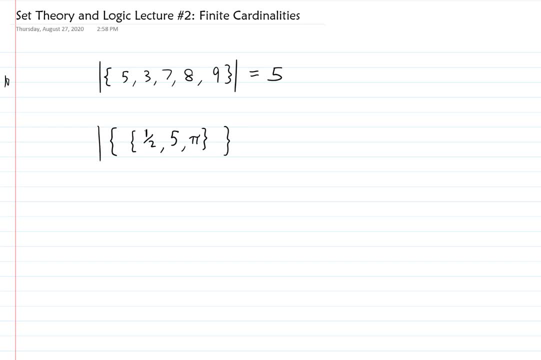 So I asked you this question: What is the cardinality of a plus one? Okay, of that. Think about it for a second Okay, And I'm going to tell you the answer. and you either got it right or you got it wrong, And it's one of these two answers. I know it. 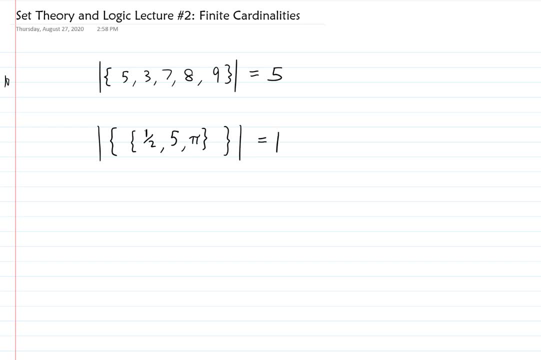 And the answer is one, Okay. Some of you said three, And that's perfectly fine to say that, But it's not correct. The answer is one, Okay, Let me show you the reason why I'm going to draw a picture here. Remember the analogy I said in the last lecture, because this analogy will help. 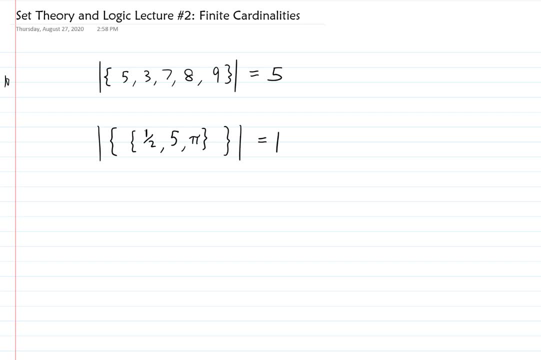 you on almost every single problem about cardinalities. Okay, And that is what is a set and what are elements? Think of a set as a cardboard box And the elements are the things that you see when you draw a picture, When you look into the box. Okay, Listen very carefully to what I said. I didn't say. 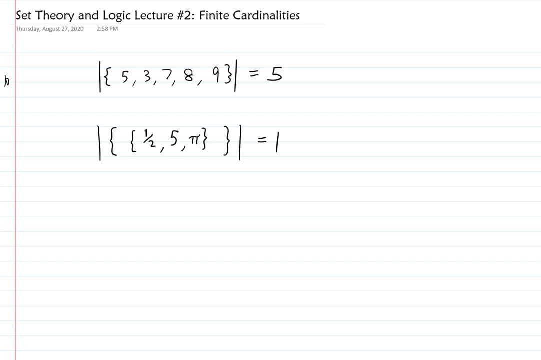 the elements are the things in the box, Although that would be true, But that's not the way I said it is it? I said the elements are the things that you see when you look into the box. Okay, So let's look at the first problem. 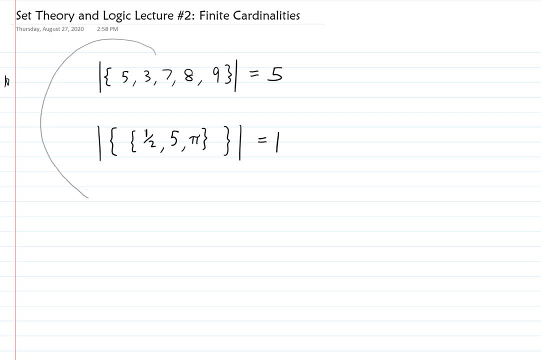 This set right here, Okay, So. So, what is that? It's a cardboard box, Okay, And inside that cardboard box are five blocks, like the kind you probably had when you were a kid. One of them's got the number five on it. 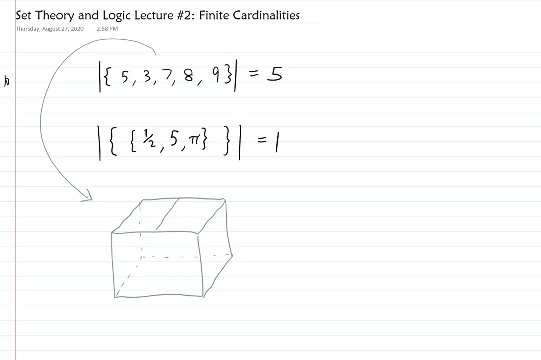 Here To save time. This is going to take us all day, So to save time, I'm just going to draw a square. Okay, That's a little block with a five on it, And there's a block in there with a three. 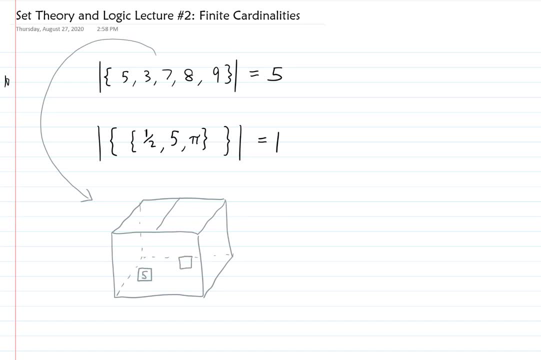 on it And there's a seven and an eight And a nine, Okay, So when I open that box and I look inside, Okay, How many things do I see? when I look down in that box, I see five things. Right, And that's why the cardinality was five. 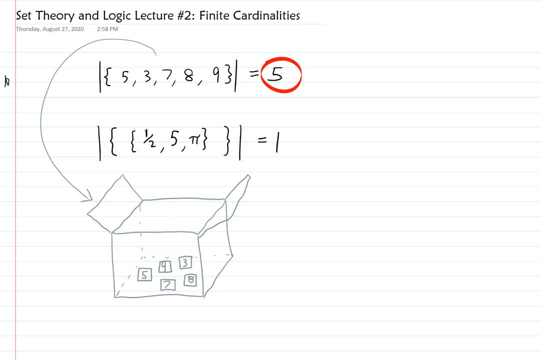 Okay, So that one is not ever Cause anybody any confusion, for the most part Okay. Now let's do the next one, And let's see why that answer is one. So what I have here? So I have a big cardboard box. 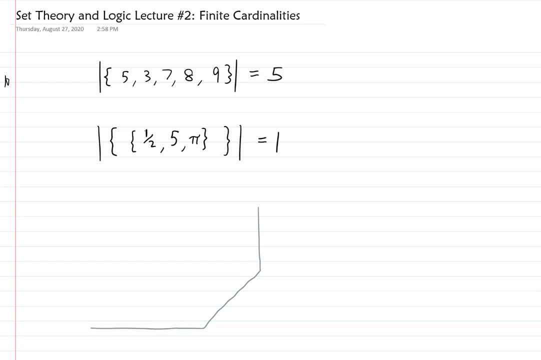 I have Here, Here, Here, Here Here. okay, there's a big cardboard box and i'm asking: how many things do you see in that box? okay, so what's in that box? in that box is a cardboard box. let me erase these dashed lines. i think we're. 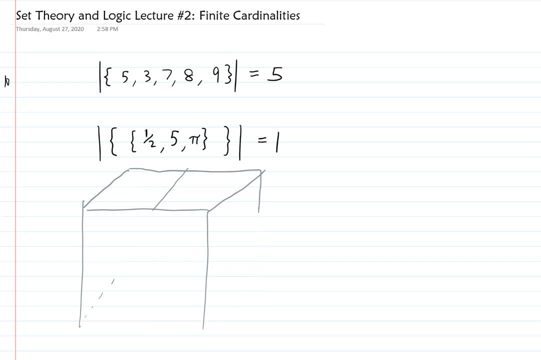 going to have too many lines in the picture. oh, i don't want to go that far, hang on, okay, there we go. okay, inside that box is another cardboard box- you see how i'm making these boxes- is closed. i'm doing that on purpose. it's like they're taped closed. okay, and inside that little. 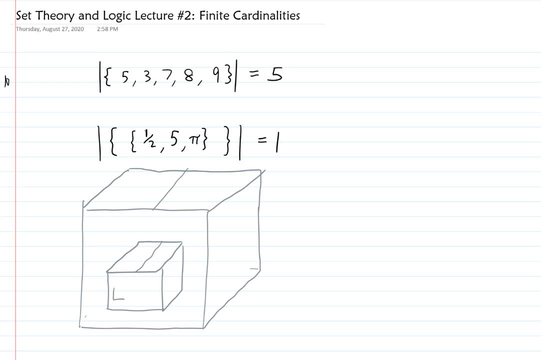 box are three numbers. there's a block with a one half and a block with a five and a block with a five. okay, now i open the big box and i look to see how many things do i see there it is again. remember i'm not saying how many things are in. 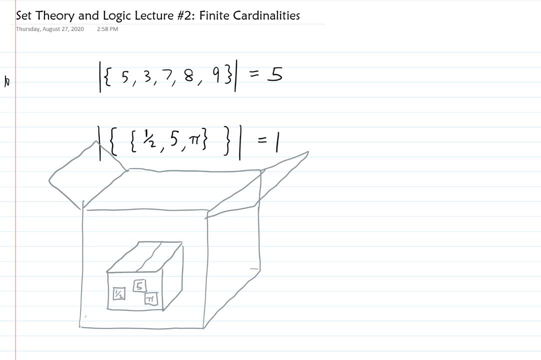 there i'm saying: how many things do you see? so look at that picture. if you look down in that box, how many things would you see? now, mind you, this is made out of cardboard, not plexiglass. you can't see through the cardboard. so when you look inside that big box, what are you going to see? 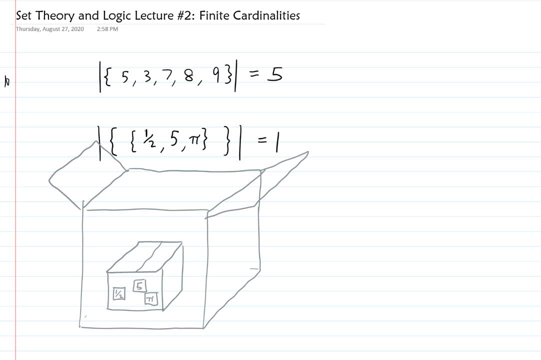 you're going to see a cardboard box that's closed. i drew it that way on purpose. right, are you going to see the one half and the five and the pie? no, because they're inside of another box and you can't see through that. you're not superman or wonder woman. 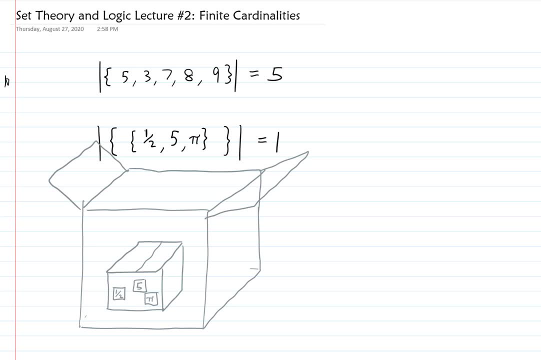 okay, so how many things do you see when you look in there? you see one, and so the cardinality of that set is one, because that's how many things you see when you look in there. okay, now the cardinality of this set, that's inside of the other set. 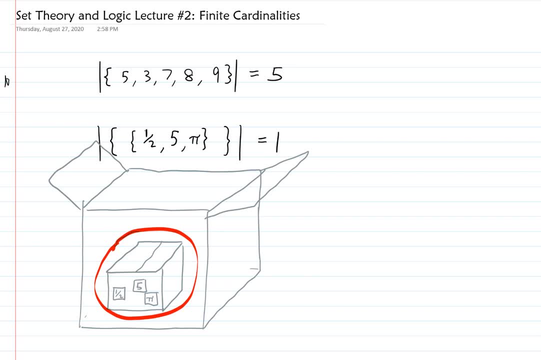 okay, the set inside has a cardinality of three, because if you opened that little box and looked inside, you would see three things. so the cardinality of the little set is three. and then that little set is inside of the bigger set and that little set is the only thing in the big set. 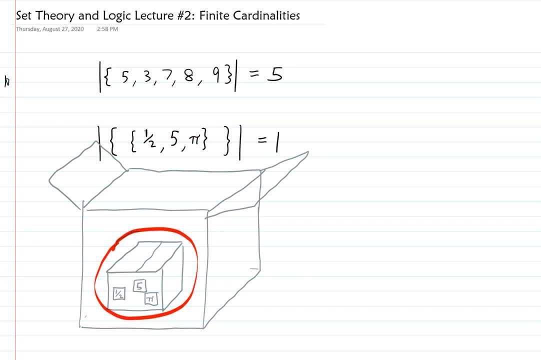 so the cardinality of the bigger set is the only thing in the big set, so the cardinality of the big set is one. Okay, I hope that makes sense. If it doesn't, you can ask me during one of the discussions, But usually the box analogy is something that will help you through any. 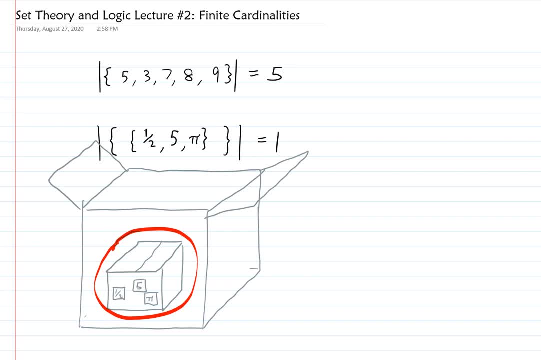 difficulty of cardinality as long as there's not infinitely many elements. Okay, All right, Let me erase that picture. So let's just do a few more. now. What if I did something like this? Here's a set that has inside of it the number 10 and a flower. 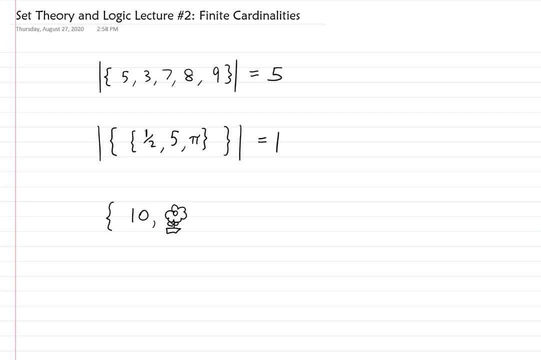 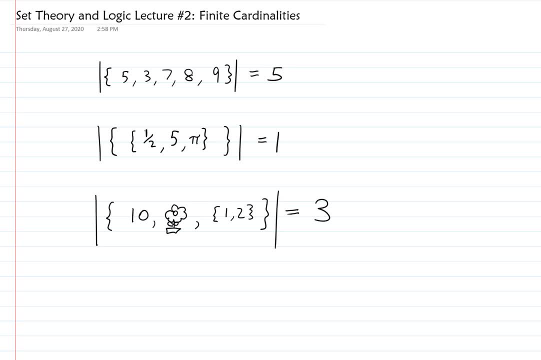 I would see a flower and I would see another box. Here's the other box, right there. Well, here, let me do it like this. So there's the number 10 that I would see, And I would see a flower And I would see another box. So I see three things. I don't see the one and the two. 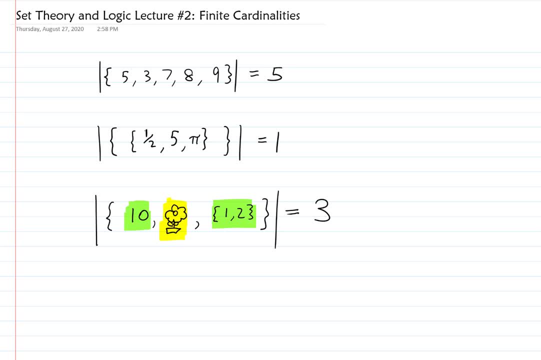 when I look inside the big set, Because the one and the two are inside of the box, Something else. Okay, It's not that hard right? It's pretty straightforward. All right, Let's talk about the empty set. Do you remember what that is? That's exactly what the name. 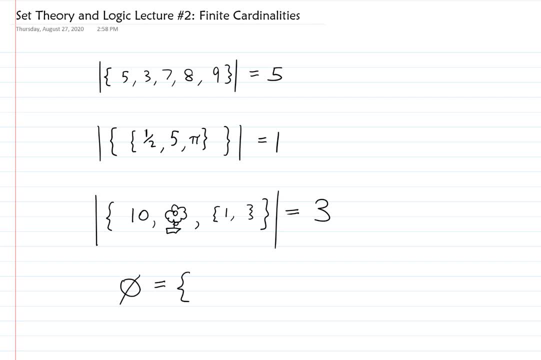 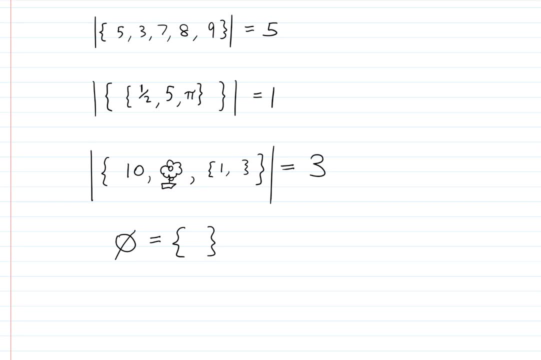 says It's an empty set. What's the cardinality of that? That's not a trick question. It's zero. The cardinality of the empty set is zero because you don't see anything in it, Because there is nothing in it. Okay, But don't get that confused with this. Oh, I see I erased that two from that. 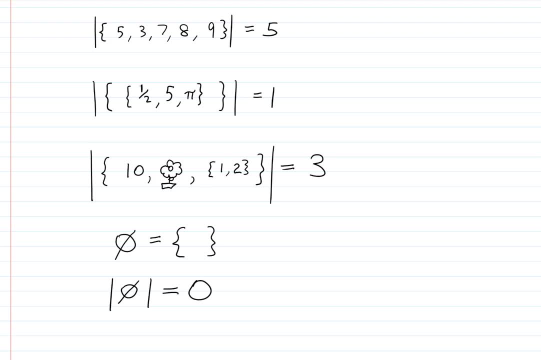 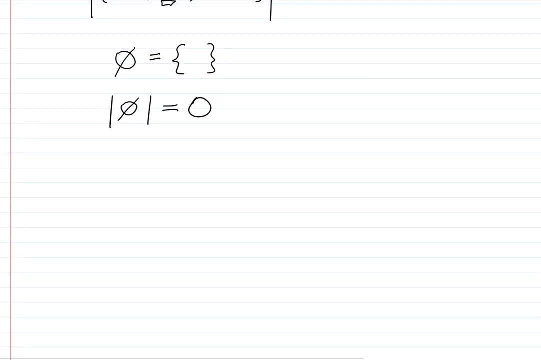 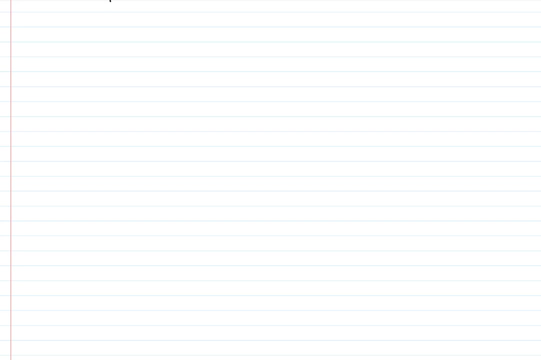 earlier problem. There we go, Don't get that confused with this. Here's a problem that we like to ask. that always confuses people the very first time, But then again, as soon as you say: oh, I understand now the mistake, then it'll never bother you again. Okay, So, because I 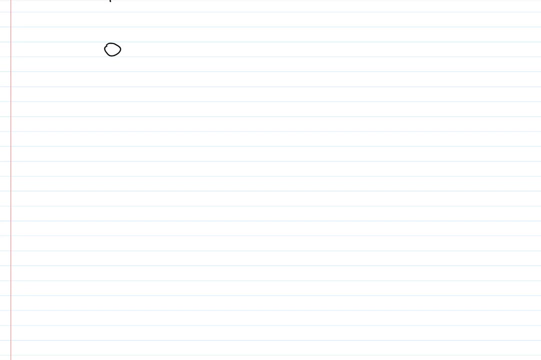 scrolled off of the screen. I'm going to just write again here. This is what the empty set is, And the cardinality is zero. Okay, Now look at this set. Okay, Is there anything in that? And if so, or if not, what's the cardinality of that set? Think about it Now. again, there's only. 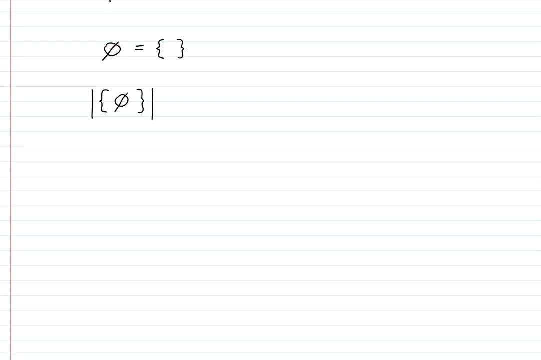 two answers that anybody ever says for this, And one of them's right and the other one's wrong. Okay, Here's the correct answer. Let me up here, let me write the cardinality of the empty set for you. The cardinality of the empty set is zero. Okay, The cardinality of this set is one, Because there's. 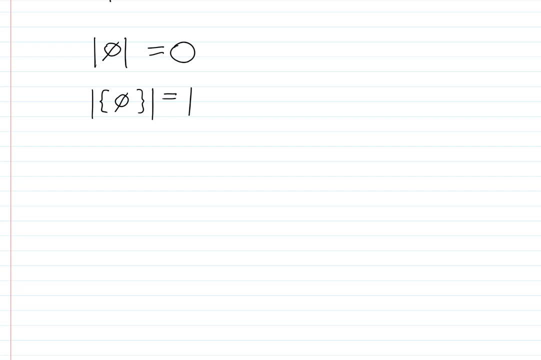 something in there. You know what's in that set? The empty set is in that set. It wouldn't make sense, would it, if I did this? I'm going to take an empty box. That's the empty set. There's nothing in there. That's the empty set, and its cardinality is zero. Okay, And that's why. 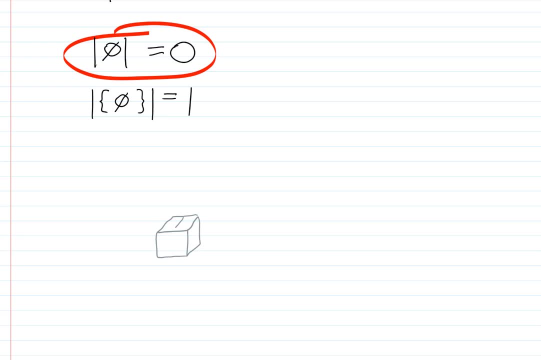 we get that up there, Okay, But now what does this say? It says it doesn't say the empty set. That's what's important. It says a set with the empty set inside of it. So my claim is that that set. 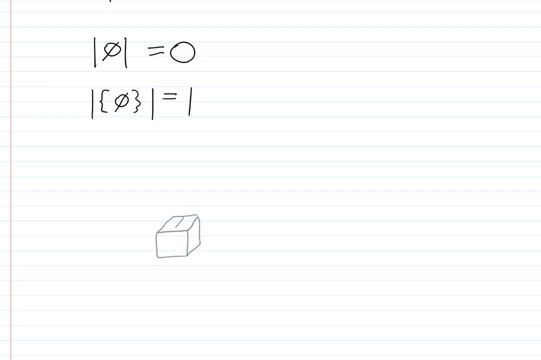 that's not empty. So let's take that empty box that I drew down there, And now I'm going to put that empty box inside of a bigger box, Tape it shut, Okay, And then I'm going to ask you to open that box and see if there's anything in it. 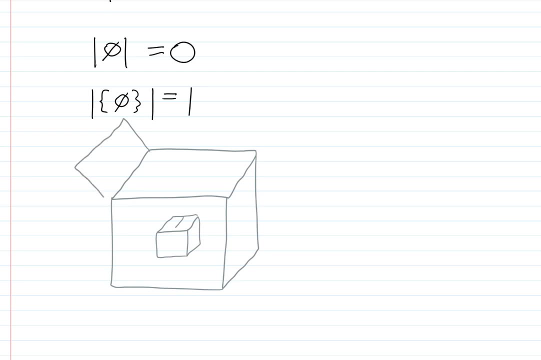 So let's open that box, Okay, And let's say: you look inside, Is there anything in there? You see, if you said no, this big box is empty, then I would say, oh, you better go to your optometrist. 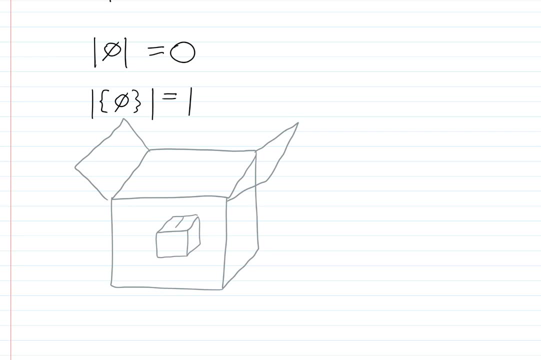 Because when I look in that box, I very clearly see that there's something in there. isn't there? Okay, This box is inside there. So you can't say that the cardinality, the cardinality of this set is zero, because that set's not empty. 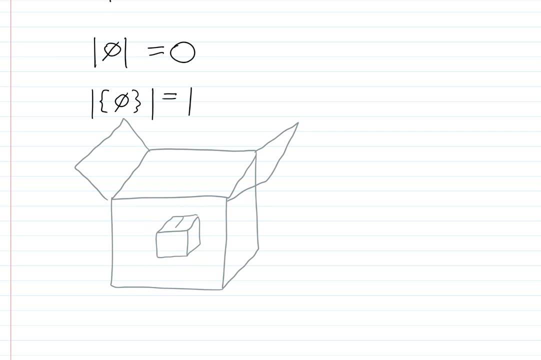 The cardinality of this set is zero. That's the empty set. Okay, But this set is not the empty set. That set has one thing inside of it, So the cardinality of that set is one thing inside of it, So one, Okay, You see how that works. 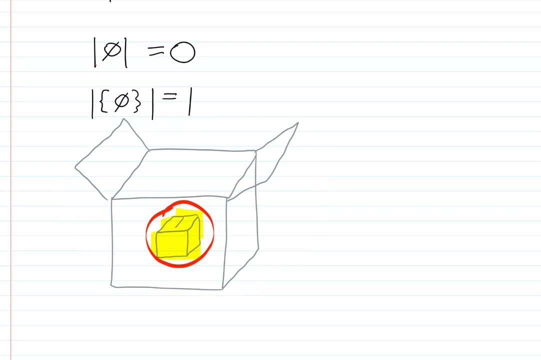 It's not confusing. It's just that almost everybody will say the wrong answer first, but then as soon as they realize, then they got it straight. It's not the sort of thing that keeps causing problems over and over again. Okay, Let's do one. just a final practice on this. 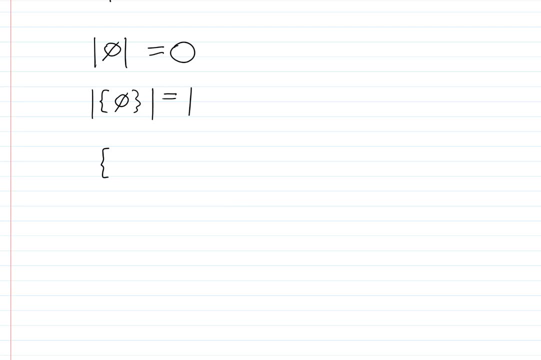 Let me write a set that has inside of it it let's say 1, and the set containing 2 and 3, and the set containing 4, and the set containing 5, and the empty set inside of there. okay, So I'm going to ask you several questions. 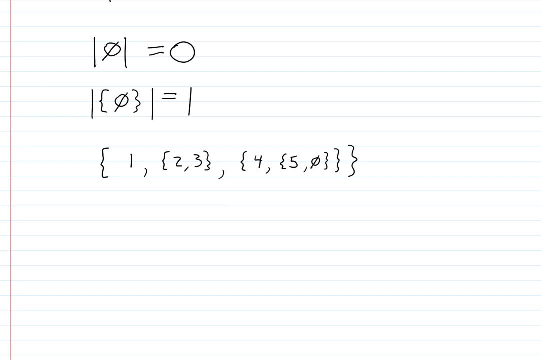 about this. okay, There's a set right there, the empty set. What's the cardinality of that? It's 0, right, Cardinality of the empty set is 0, okay, Now let me ask you a new question. 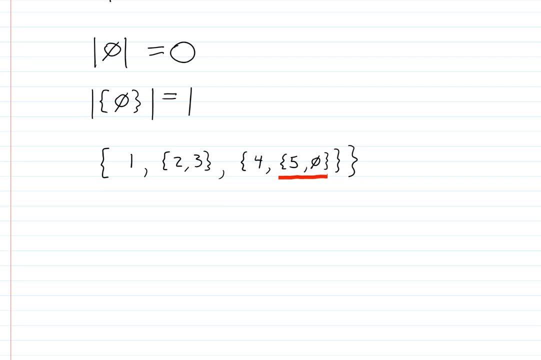 Here's another set. What's the cardinality of that? Okay, I hope you say it's 2, because that's correct. That set has a 5 and the empty set or the elements, okay, So that cardinality is 2.. Now here's a bigger set. 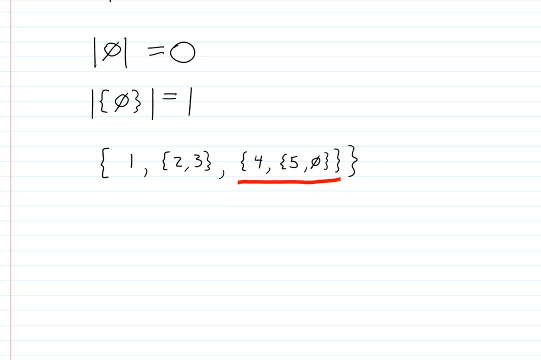 What's the cardinality? The cardinality of that Careful, Don't be too quick to answer, okay, Carefully. You know how many things I see in there. I see a 4. That's one thing, And I also see this. 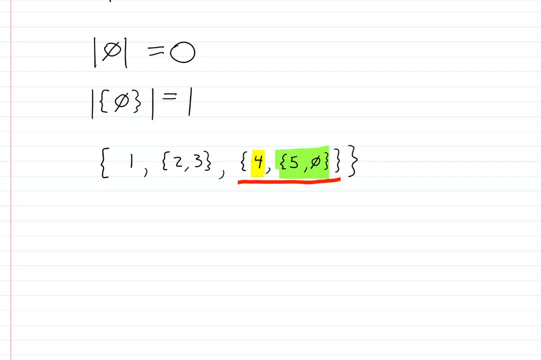 set. I see two things in there, Not three, just two, Because when I look in this set that I've underlined in red here, when I look in that I don't see that 5 and that empty set. I don't see that 5 and that empty set. I don't see that 5 and that empty set. 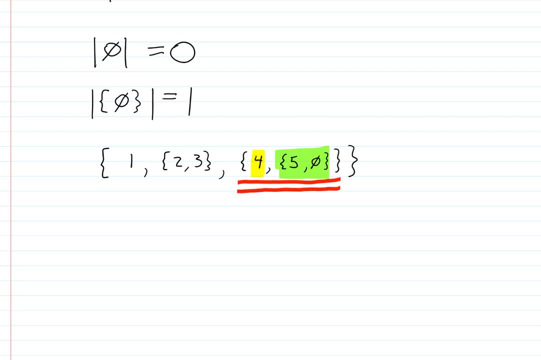 Because they're inside of a smaller box. I can't see through the cardboard of that smaller box. Okay, do you see what I'm saying? All right, let's move over. Here's another set here. That one's a little bit easier. What's the cardinality of that? That's 2.. 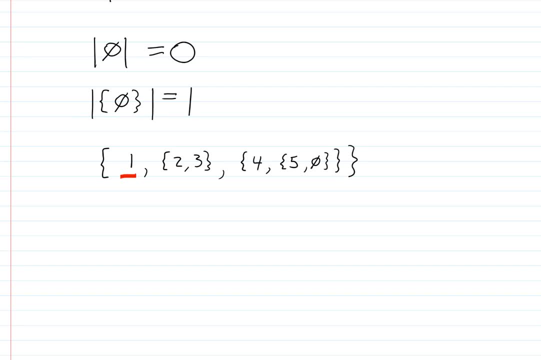 Is that a set? No, that's not a set, is it? There's no curly brackets. All right now final question, and this is the big one: What's the cardinality of that set here? Well, let's see. How many things do we see? Let's count them. I'll circle them in purple. 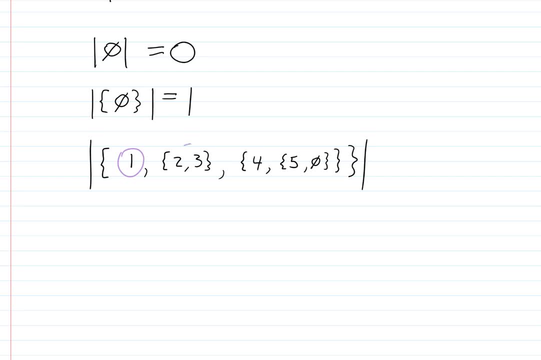 There's one thing here. I'll circle them in purple. I'll circle them in purple. I'll circle them in purple. There's one thing that I see, Here's another, And here's another. How many things do I see? 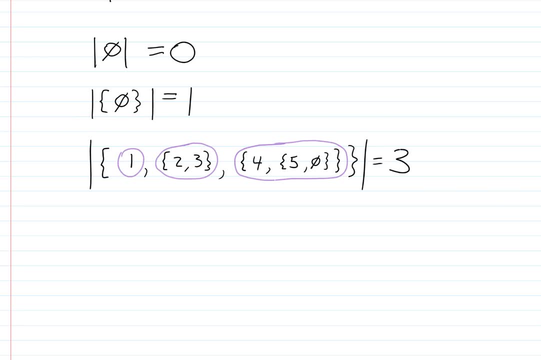 I see 3.. The cardinality is 3.. By the way, you might notice this. Look, You can also use the commas to help you count that. There's two commas, so that means how many things are being separated? Three things, And why would I not count this? I don't know, I don't. 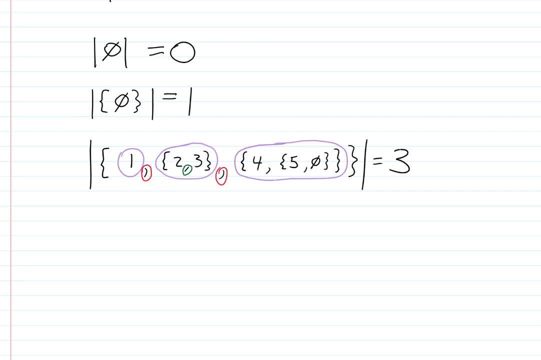 count this comma because that belongs to these brackets, You see? So that's not a comma for the big set, That's a comma for that smaller set. You see what I'm saying? Same thing here. I wouldn't count this comma because it belongs inside of these brackets. So that's for that. 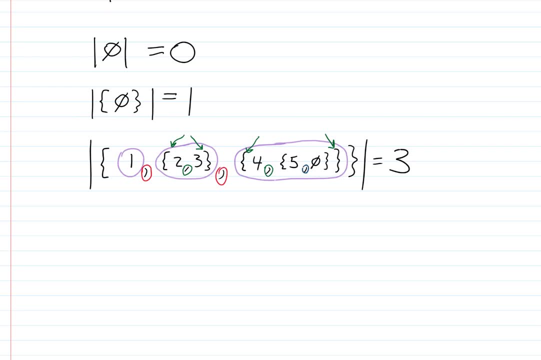 smaller set And I wouldn't count this comma because that is for this set. The only commas for the big set are the ones I circled in red, And there's two of them. Two commas means three elements. Okay, All right. Now I just want to do a little bit of practice with set. 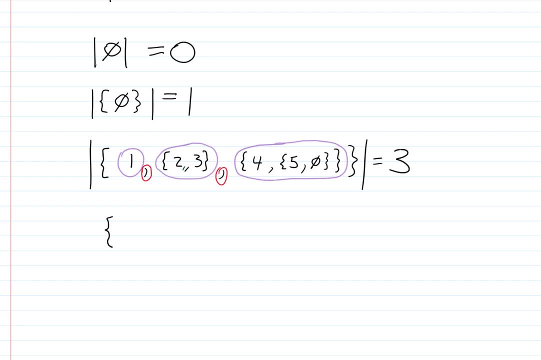 builder notation. We went over that in lecture one. What if I wrote this: The set of all x in the integers, such that x- sorry, x- squared, is between 10 and 100.. Okay, And the question I want to ask is: what's the cardinality of that set? Okay, So I'll. 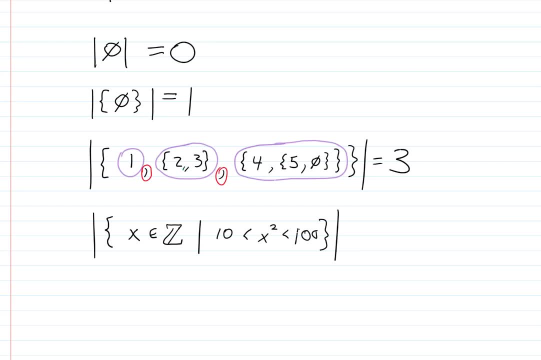 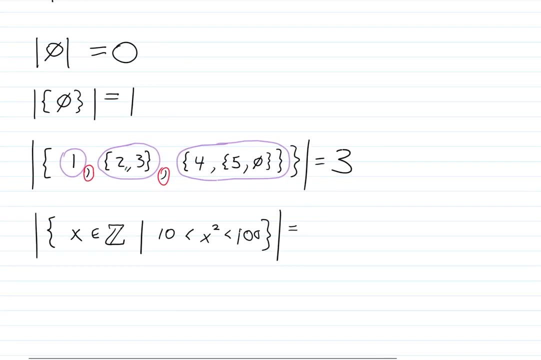 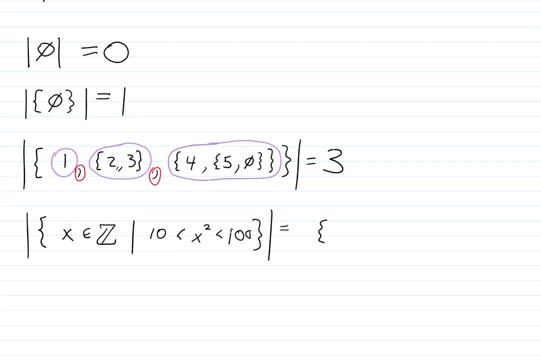 give you some advice. How about if we just rewrite that set by listing the elements, Because I don't think there's going to be all that many, So that set would really just be what Let's see. Two squared is four, so that's not going to be in there. 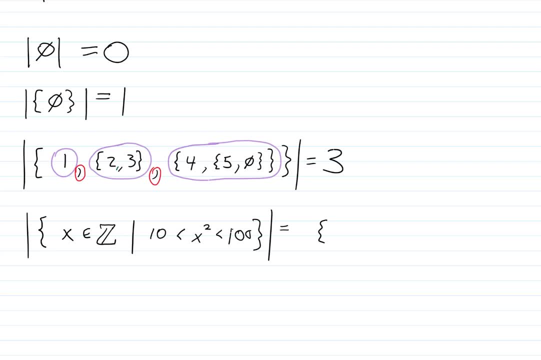 Three squared is nine, so that's not going to be in there. Four squared is 16, that'll be in there. Five squared is 25, that's between 10 and 100.. What else will be in there? Six will be in there, because six squared is 36.. Seven and eight and nine will be in there.